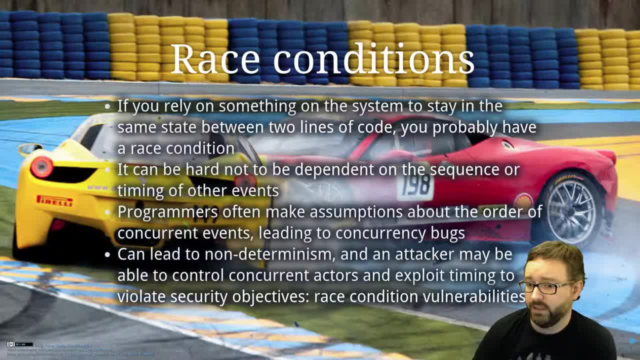 race conditions and concurrency bugs, essentially, So it can lead to non-determinism. So basically what we want, we want things to be deterministic. usually when we're talking about things happening on a computer, We kind of want it to be predictable: This happens, and then this happens, and 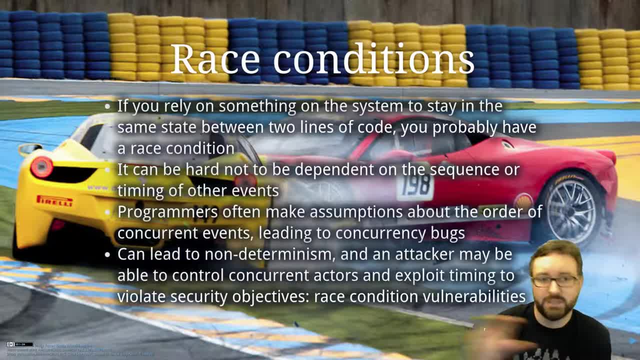 always results in this, But if there are things happening in between what we're trying to do. so you know, our code does this, and then it does this, and then it does this, but in the meantime, while we're doing that, someone else on the computer deletes a file or accesses a file or changes the contents. 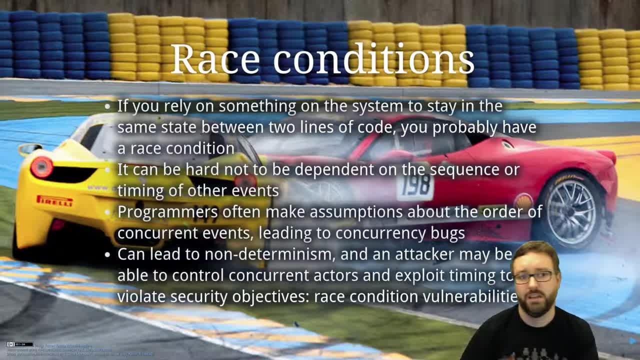 of a file between our actions, of our software, then that can lead to race conditions. So we might, you know actors, so the attacker might be able to actually control some of the concurrent actors, whether that's just processes happening or threads within a program, and exploit the timing to violate security. 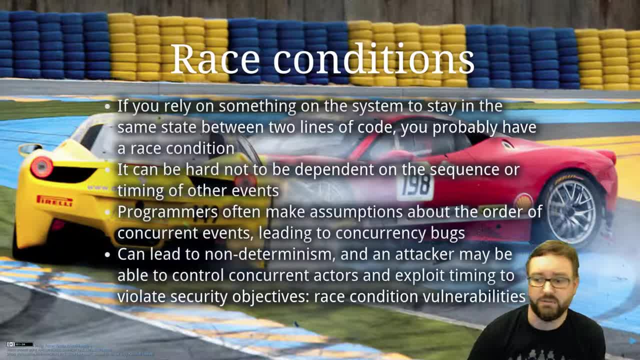 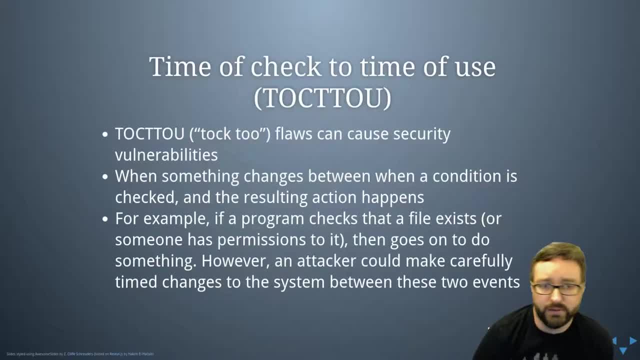 objectives And if they can do that, then that is a race condition vulnerability. So the one of the most common kinds of race condition vulnerability is a time-of-check to time-of-use or a top-to vulnerability, and that can. basically, it happens when something changes between when we check a 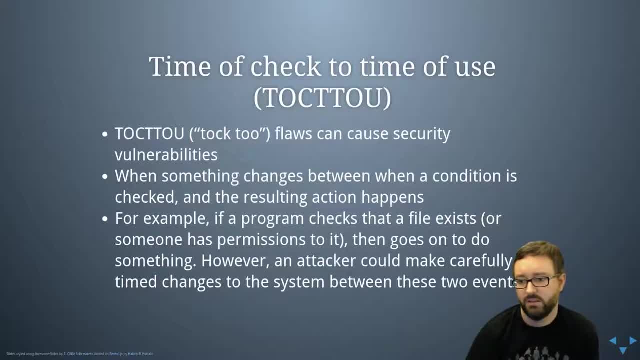 condition and then we have our resulting action. So, for example, if a program checks that a file exists or someone has submission to it and then as a separate instruction, the computer then does something, an attacker could be really careful or carefully timed, or may just spam the system trying to access a. 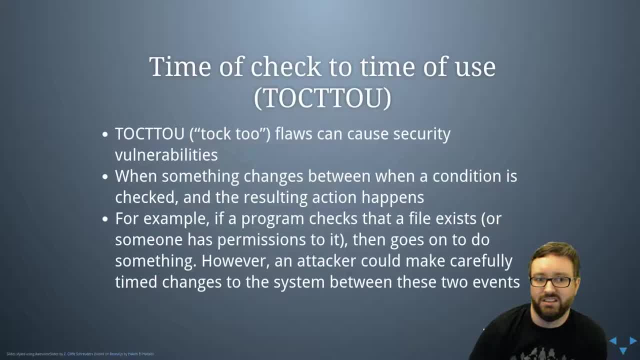 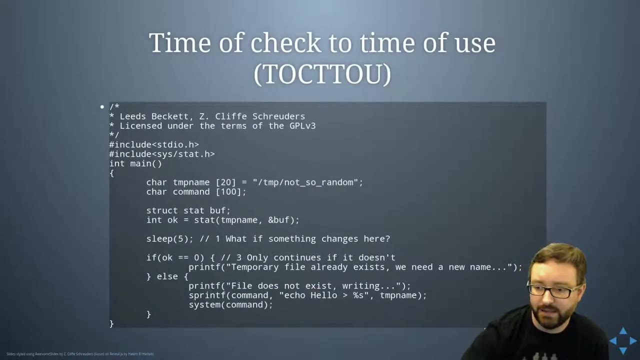 thing so that in between those two instructions executing, the attackers are able to do something That can completely violate the way that we intend our software to work and the security decision logic and everything to work. So here's an example. So in this example we have our temporary file and in this example it works best if it's. 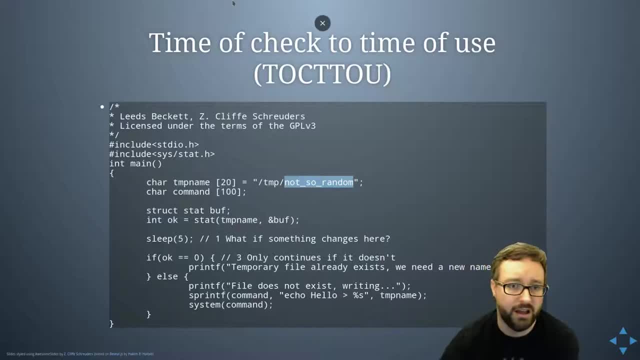 predictable, So if the attacker is able to predict what this file name is. so we've got a temp file in the temp file directory, called not so random, and we've got a command variable. we've got a stat structure, which a structure is like a. well, in C programming a structure is a. 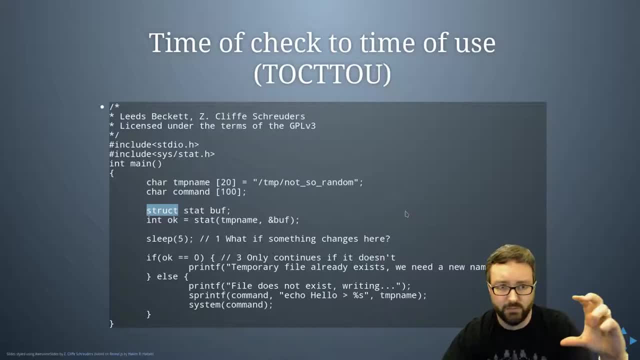 variable that holds basically multiple data types in one loop area of memory And basically we do a stat on the file name, And stat is a function that gives you information about a file. In this case we've got a busy program. There's lots of stuff happening in this code. 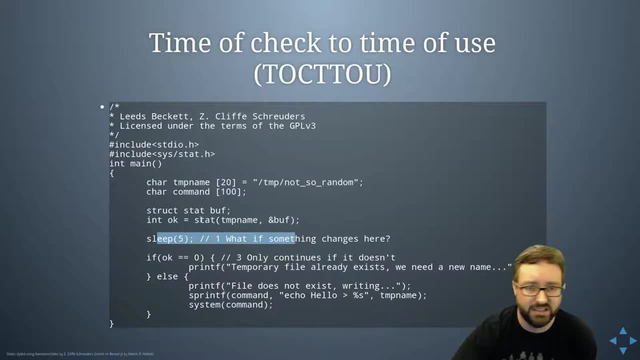 You didn't actually have to sleep, but this is just exaggerating. Something else is happening in our program, But then we check whether or not it was OK. So you know, does the file exist? And if it doesn't exist? so if a file already exists, then we'll just print an error message. 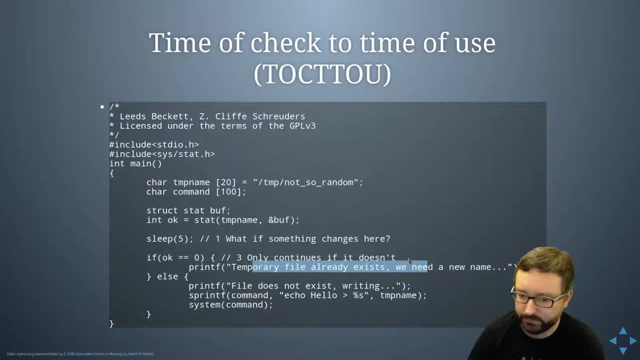 Say: you know, sorry, something's gone wrong. If the file doesn't exist, then we're going to create it, And in this case we're just sending a bash command that says hello, and it stores it in the file. And now the vulnerability here is that. 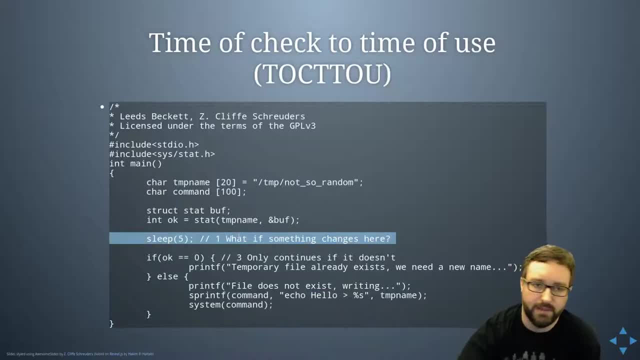 while the program's sleeping, or even if we didn't have that command just in the time, this fraction that it takes between us checking and then doing. if they go and create the file, then our content gets put into that file that someone else now owns and has the ability to set the permissions for, for example, 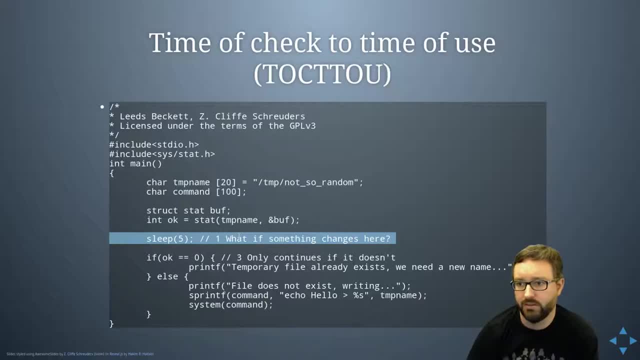 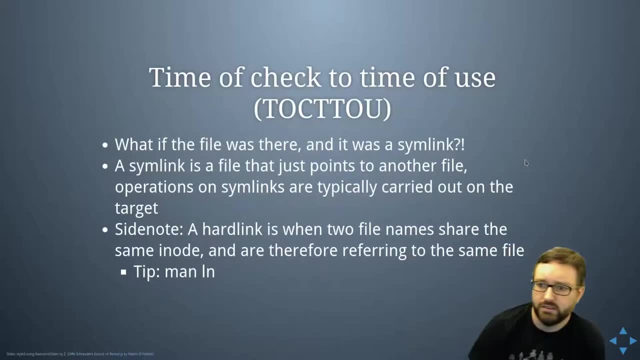 So there's a classic example of a TOC2 time of check to time of use security vulnerability, which is a rarity. It's a race condition, So you know what other file is there And it was a symlink. So a symlink is a file that just points to another file. 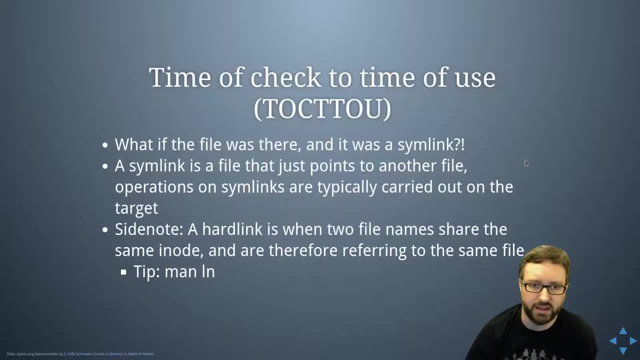 And operations on symlinks are typically carried out on the target And you know, as you will probably be aware, hardlink is when you've got two names that share the same inode and therefore they're referring to the exact same file. 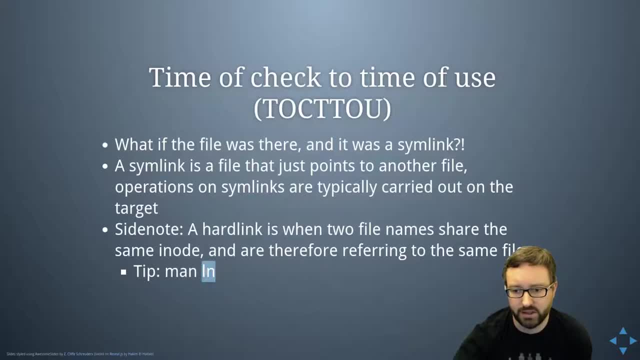 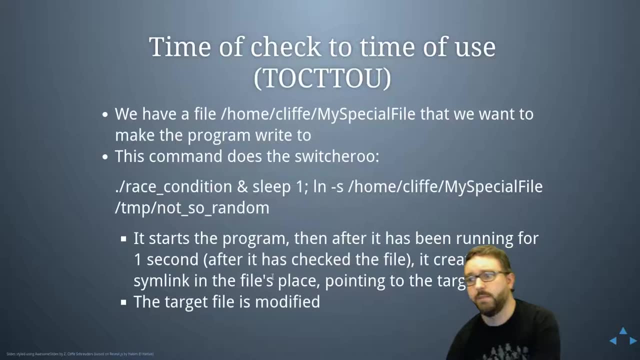 And if you want to read a bit more about that stuff, you can type in manln, which will give you the man page for the link command. And so we've got a file that we want to make the program write to, And so this is an attack against that code that we just saw. 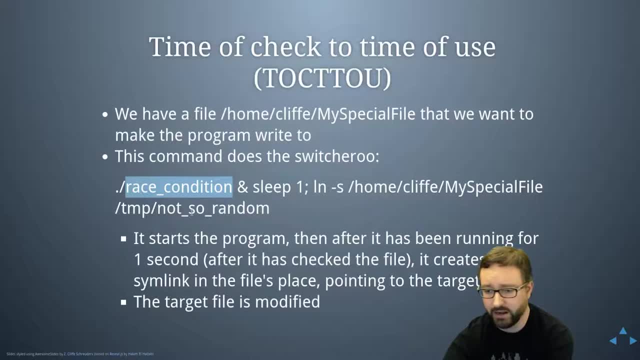 We can, basically, when the race condition program is running, we just have to kind of time our attack so that while that is in between its instructions, while it's doing its sleep five command, So we just kind of like start the program. Wait a second. 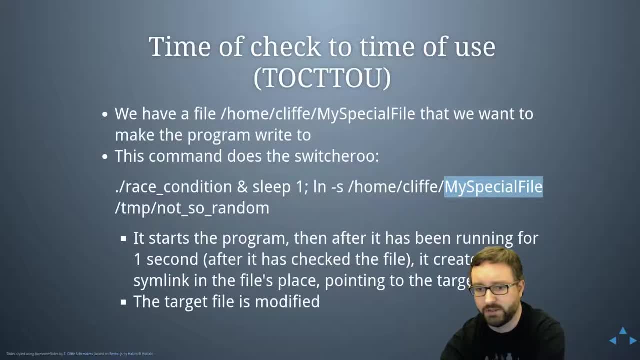 And then we create a link to my special file from the not so random location And then it's already checked whether that file exists. It's decided it didn't exist. It then writes the file and it writes it into my file Could even wouldn't even need to create a link. 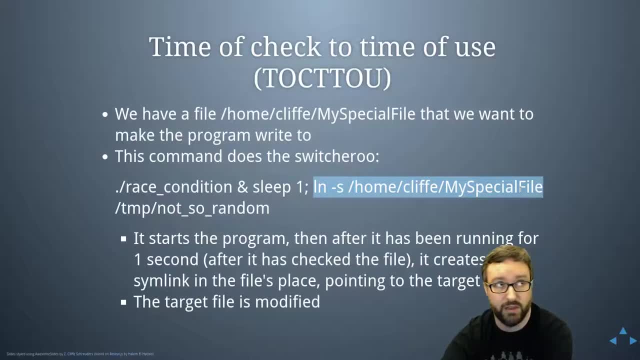 We could just actually create a file. As long as the as long as that user has access, has the permission to write to the file, then it would work as a way of basically getting him to put the content into our file rather than a file. 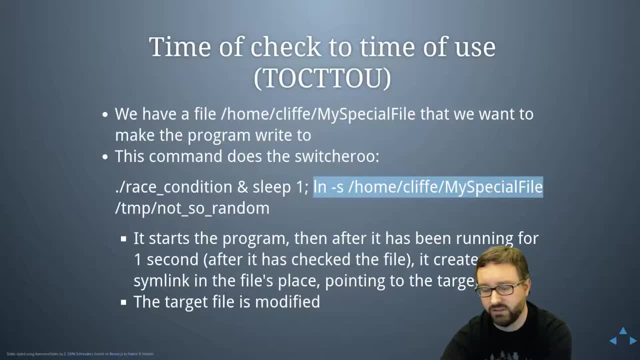 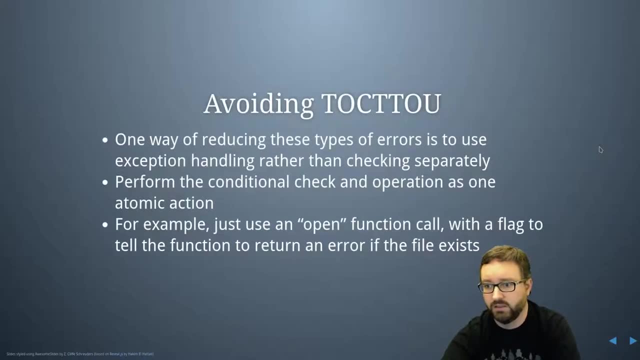 a temporary file that it owns and can set permissions on. So Yeah, bad news. So the way that we can reduce these kinds of errors is to use exception handling. So, rather than doing a check and then as a separate instruction where you take the action, 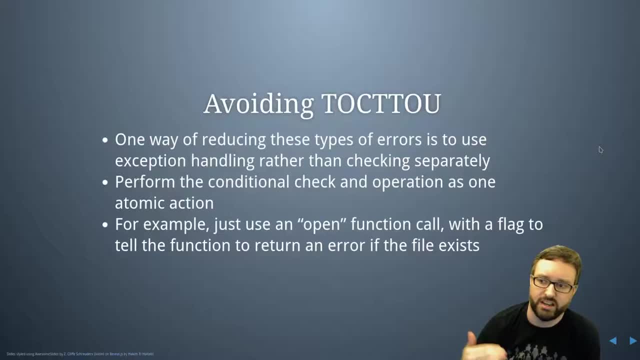 we need to be able to perform the conditional check and the operation as one atomic action. So, for example, just use an open function call with a flag to the call to say to return an error if the file exists, because then the operating system kernel provides a way for that all to happen as one action, so that nothing can happen in between. 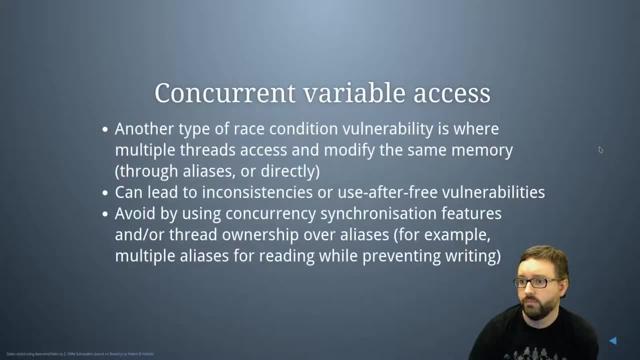 So another kind of race condition, which I alluded to at the start, is where we've actually got multiple threads of the same program that are trying to access and modify the same memory, So like for a variable, for example, and it might be through aliases. 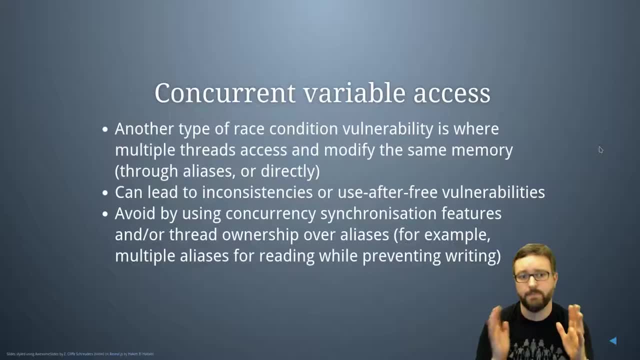 So, for example, we've got a piece of software and it has, say, five threads that are running and they're all um interested in one variable that's set for that program. If they um start accessing that variable and maybe you do something that tells it to basically delete that variable. 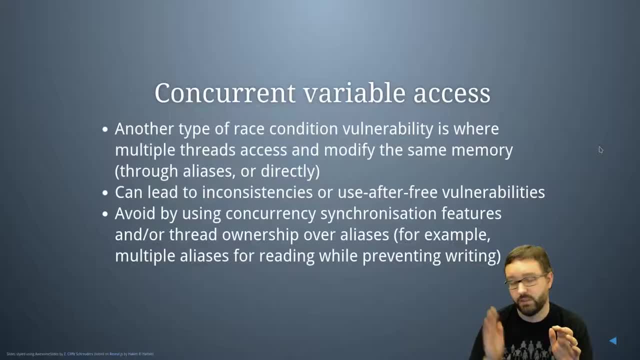 then these other other um threads might still try and read to or write to that um freed memory, which would obviously be a problem. Uh, at, at best it'll crash the program, At worst there'll be some vulnerability that allows. 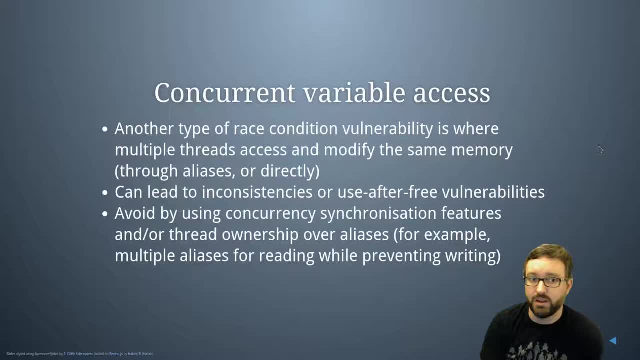 uh, a hacker to inject, um, something else into that memory, um, which changes the behavior of the code, um, of what these, you know, other threads are doing, Um, and there can. so there can be all kinds of problems with the timing of that. 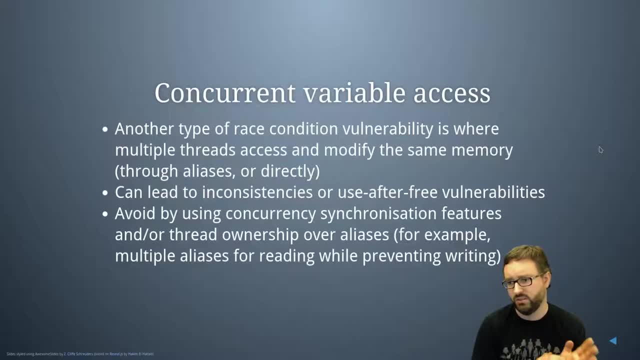 Uh, so it can lead to consist inconsistencies or use after free vulnerabilities. There are loads of um synchronization features, uh, mutexes and all sorts of like ways of doing locking, And it's a whole area of computer science um. 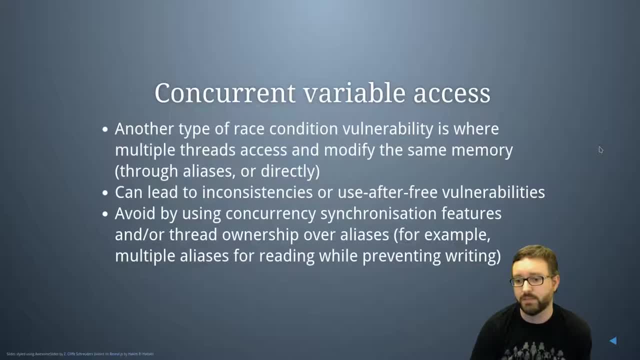 so that you know there are plenty of people thinking about this stuff. but from a security perspective, there are, you know. you just have to make sure you're doing it properly, basically to, um, avoid security problems. So there's the idea of ownership. 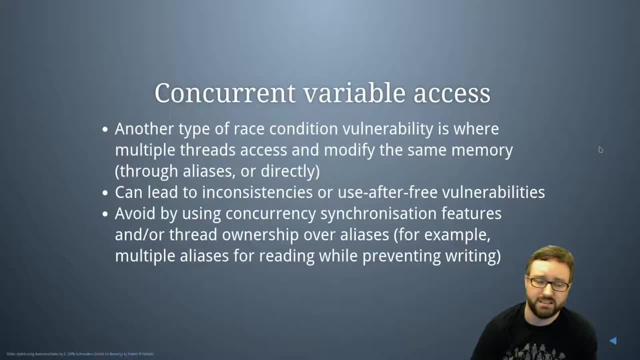 um over aliases. So if you do have a single bit of memory that's being accessed from multiple places, make one specific thread, for example, take ownership over it. So one way of doing that is to have like, uh, if you've got someone performing a right action. 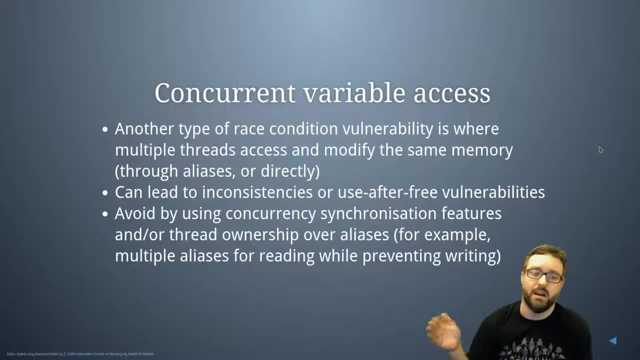 you might allow other people to read it. Uh sorry, while the right action is happening, you might let. no, no one do anything to it. While there's no right action taking place, you might say: well, all the threads can read from it. 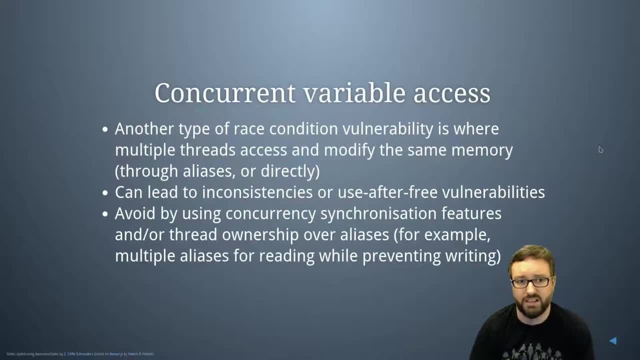 Um, but as soon as someone says they want to write to it, no one else is allowed to start reading from it. Uh, so you know, there are. there are um, all kinds of um like techniques, uh.